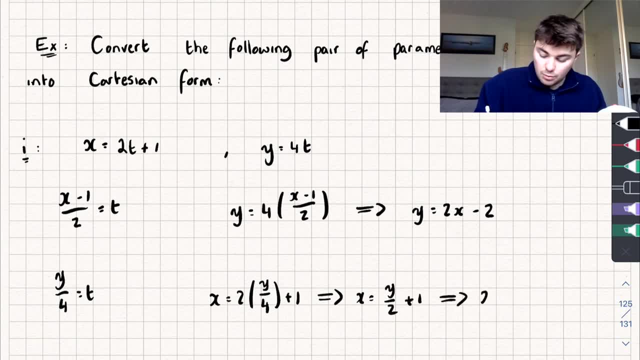 to y divided by 2 plus 1.. And multiplying through by 2, we get that 2x is equal to y plus 2, which is the same as the equation above, just in a slightly different form. So that's the first case which is. 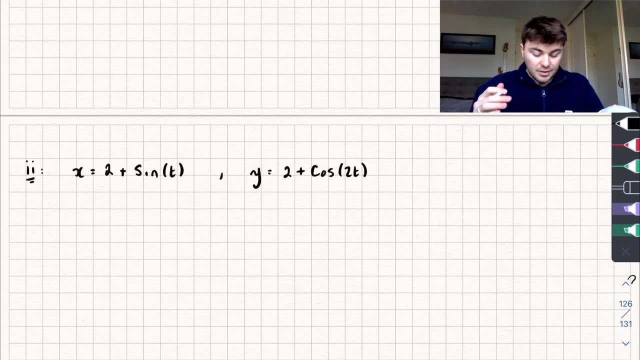 probably the most simple. The second one is slightly trickier and this is where we have sort of like trig functions in our equations. So we've got x equals 2, plus sine of t and y is equal to 2t, And so we could rearrange to make t the subject. say for the first equation, x equals 2. 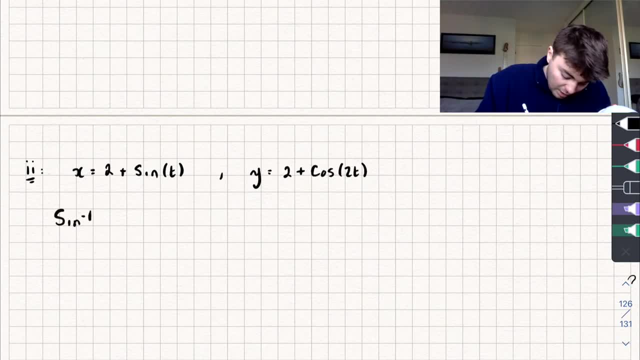 plus sine of t, But we would get that the inverse sine of x, subtract 2 is equal to t And substituting that in doesn't really make a nice equation that we want to deal with. But what we could do okay is we could substitute in sine of t into the other equation, because that's still removing our 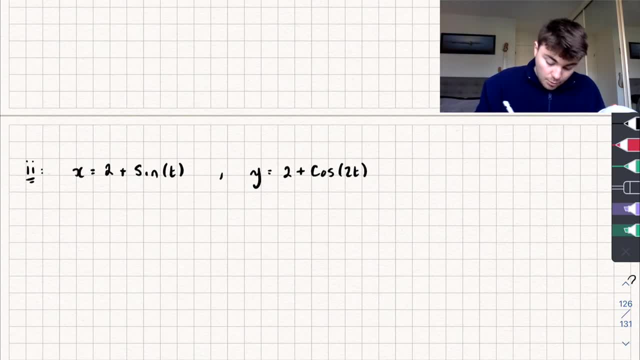 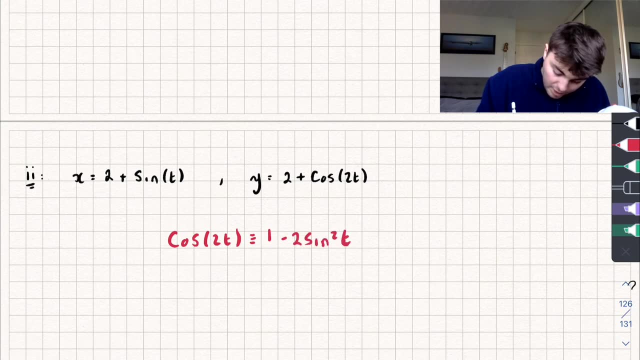 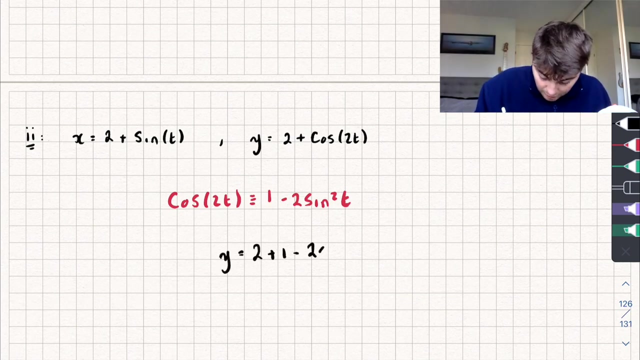 parameter, And so the way we could do that is by using a trig identity. We could say that, well, because of 2t is actually identical to 1 subtract 2, lots of sine squared of t, And so, using that to rewrite our equation for y, we get that y is now equal to 2 plus 1 subtract 2 sine squared of t. 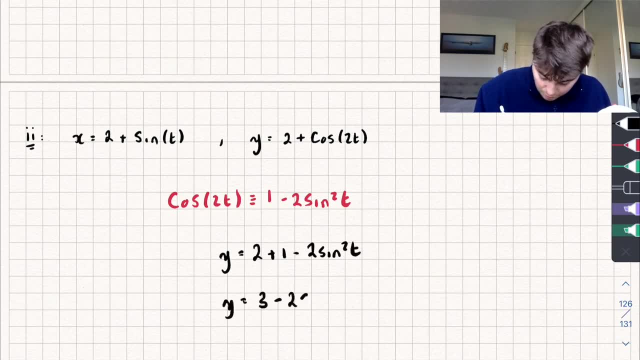 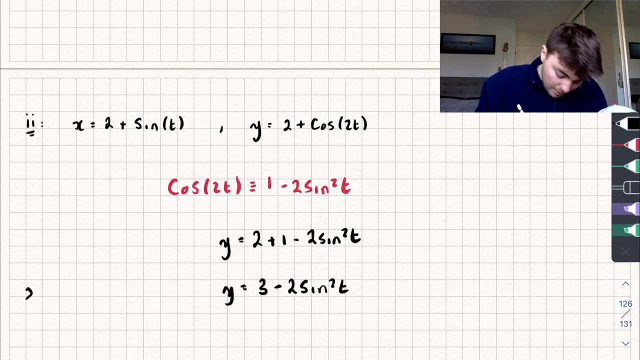 which is, if we neaten it up, y is equal to 3 subtract 2 sine squared t. Now if we rearrange our equation for x to make sine of t the subject, we get that x subtract 2 is equal to sine of t. 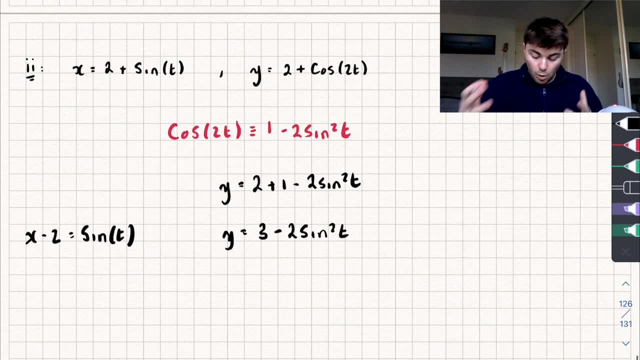 And now we can substitute in sine of t, And so we get that x equals 2 plus 1 subtract, 2 sine squared of t. We can substitute sine of t into our equation for y And we get now: y is equal to 3 subtract. 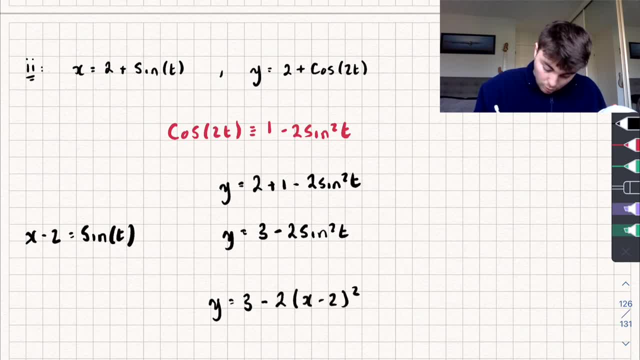 2, lots of x, subtract 2, all squared, And you can see we've now written it into our Cartesian equation form. So again, it's not that difficult. You just need to maybe use some trig identities that you know. Let's now look at the third type, okay, which is again slightly different, And so: 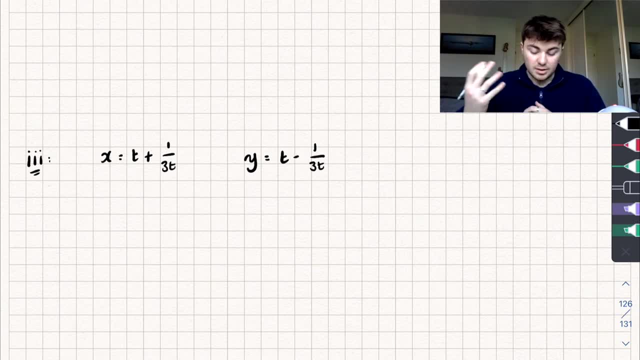 we've got x is equal to t plus 1 over 3t, And y is equal to t subtract 1 over 3t, And so, rearranging this to make t the subject, we get that y is equal to x plus 1 over 3t, And so we've got x is equal to. 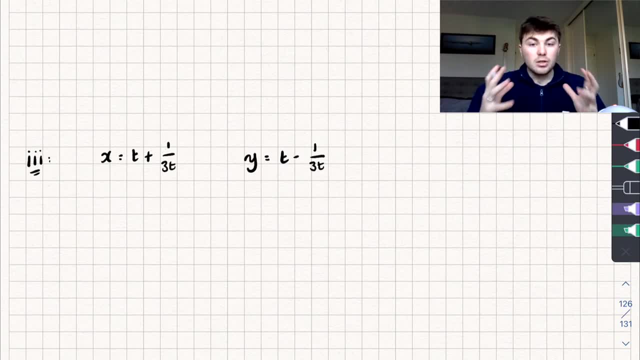 subject is going to be pretty tricky to do, and so what we could do is treat them like simultaneous equations and add them together, and let's see what happens when we do that. Well, if we add them, we get that x plus y is going to be equal to t.